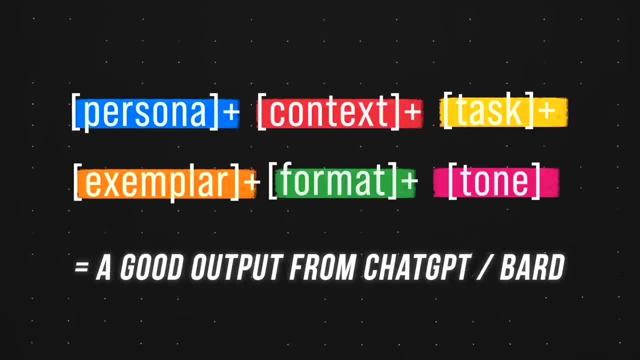 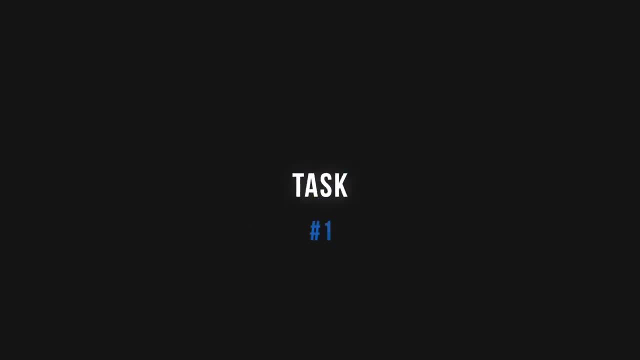 when writing prompts And, as you'll see in this next part, you do not need all six components in every prompt to have a good output. Now let's break down each building block with specific examples, starting with the task. The rule of thumb is to always start the task sentence with: 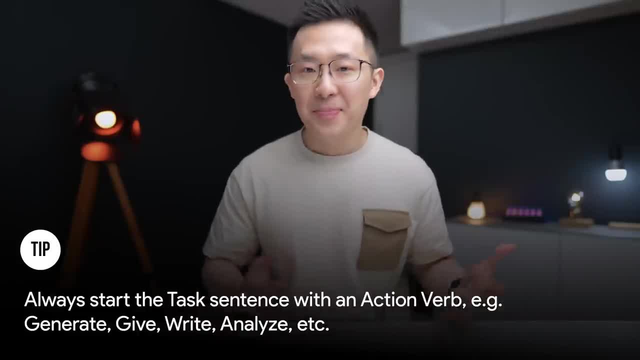 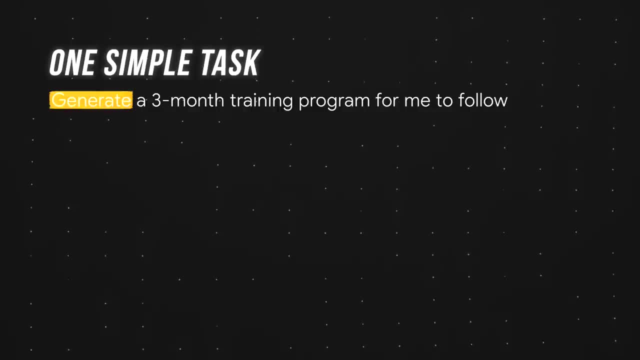 an action verb- Generate, give, write, analyze, et cetera- and clearly articulate what your end goal is. It could be one simple task, like generating a three-month training program, or a complex three-step task like analyzing hundreds of user feedback. 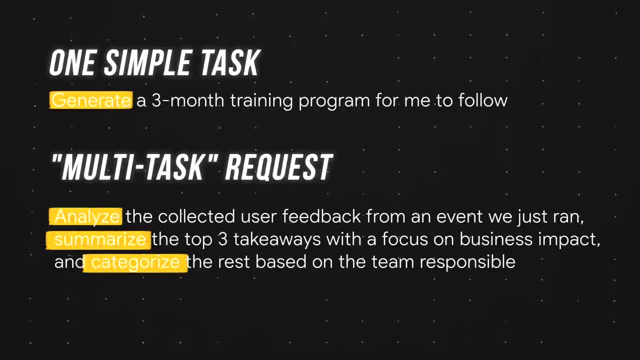 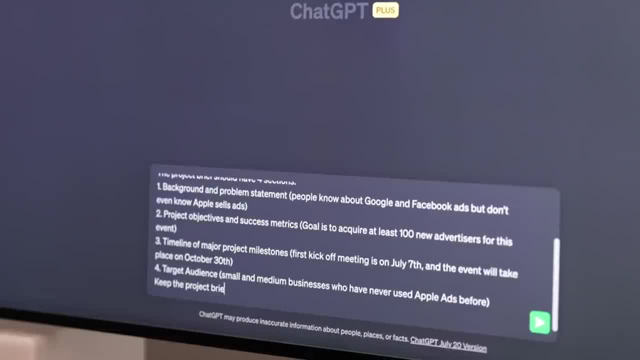 sharing the top three takeaways and categorizing the feedback based on the team responsible for following up. The second component, context, is the trickiest to get right because technically there's an infinite amount of information you can give. So I found asking myself these three. 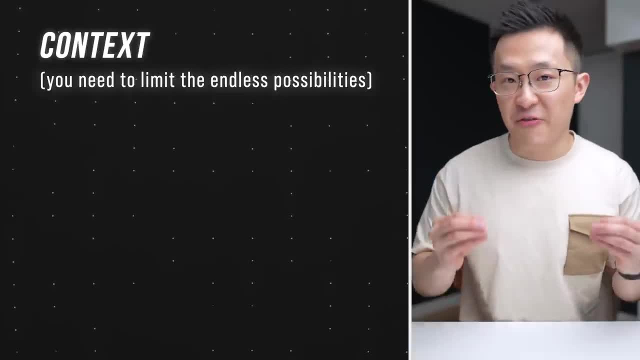 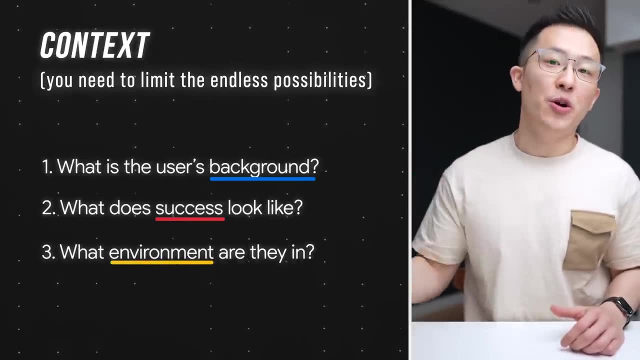 questions to be super helpful in coming up with just enough information to get a good result from ChatGPT. First, what's the user's background? Second, what does success look like? And third, what environment are they in? Back to the workout example we now have: I'm a 70-kg male looking to put 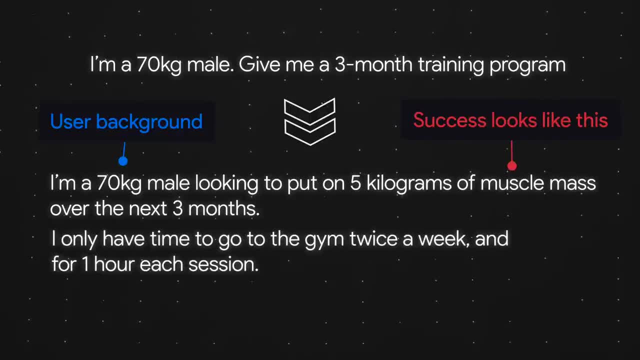 on five kilograms of muscle mass over the next three months. I only have time to go to the gym twice a week and for one hour each session, giving me a three-month training program to follow. Could I have added more background information? Of course, Only prioritize the muscle groups that. 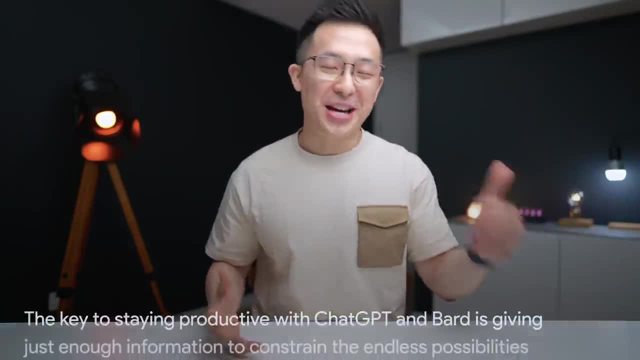 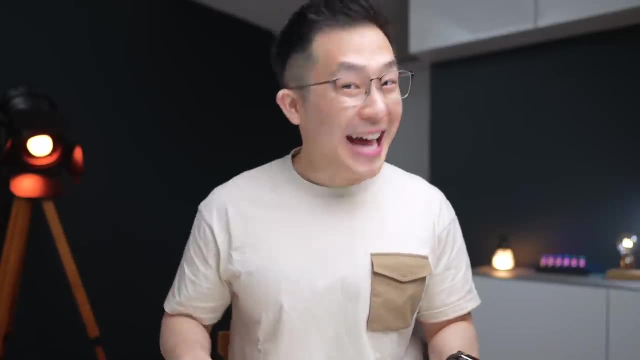 make me look good on Instagram, But the key to staying productive with ChatGPT and BARD is giving just enough information to constrain the endless possibilities. By the way, although this video is not the end of the video, I hope you enjoyed it. If you did, make sure to hit the like button. 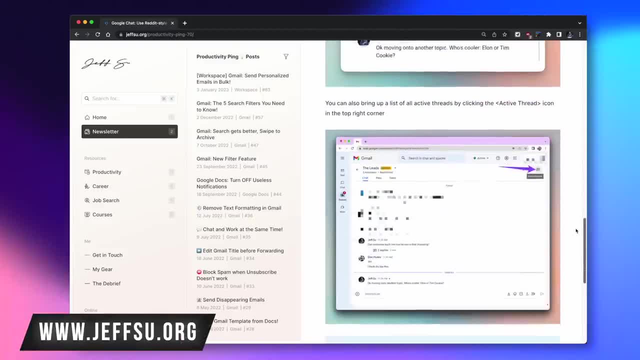 share this video with your friends and subscribe to my channel. It's free And, if you haven't, it's supported by those of you who subscribe to my paid productivity newsletter on Google Workspace tips. Link in the description to learn more. Moving over to the exemplars component, 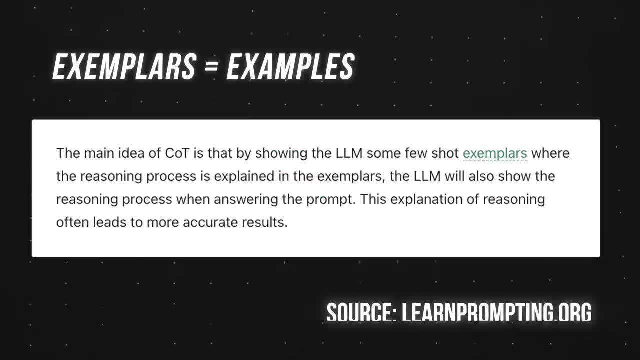 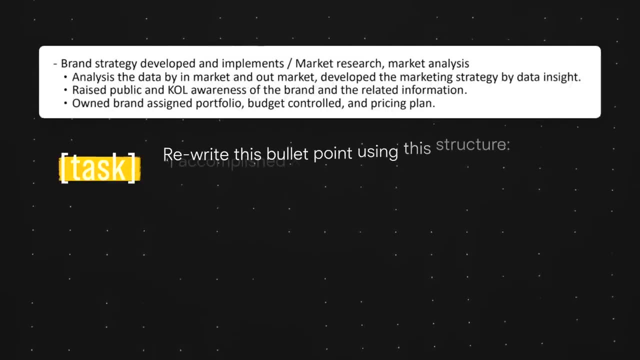 it's just a fancy way of saying examples. Basically, all the research on large language models, LLMs- have shown that including examples within the prompt drastically improves the quality of the output. Starting with a simple example, this is a poorly written bullet point from a 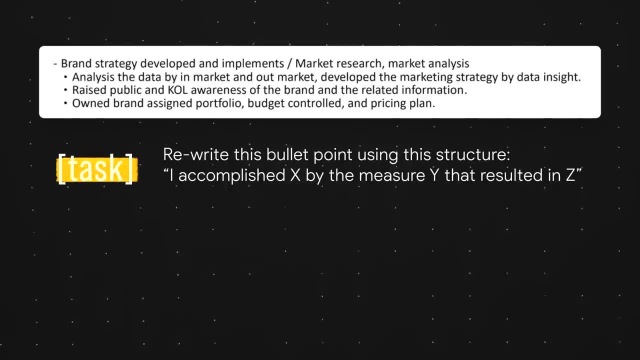 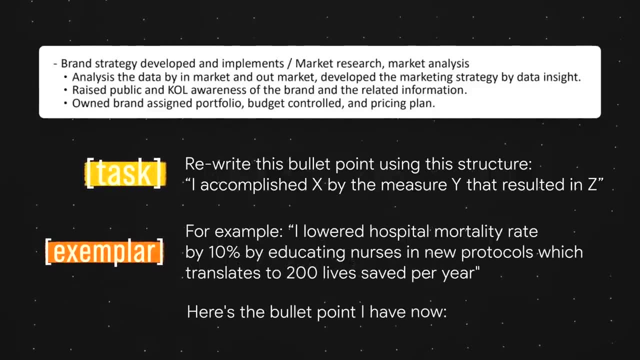 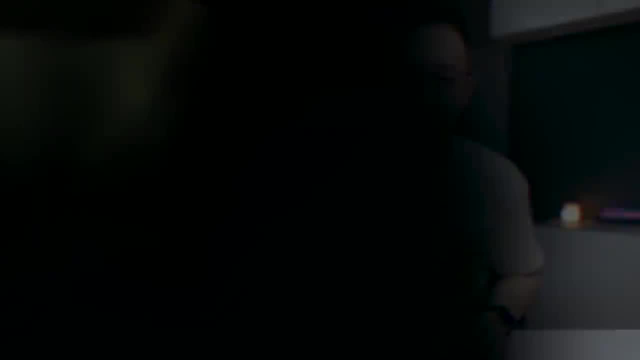 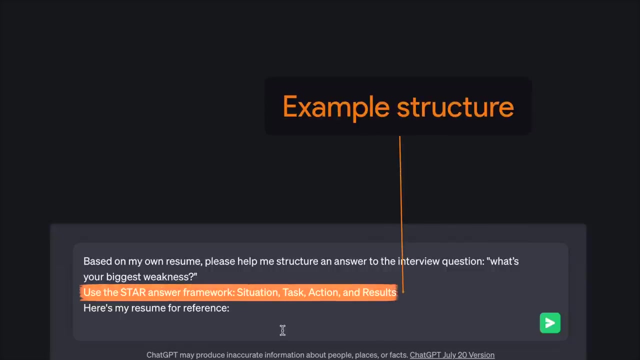 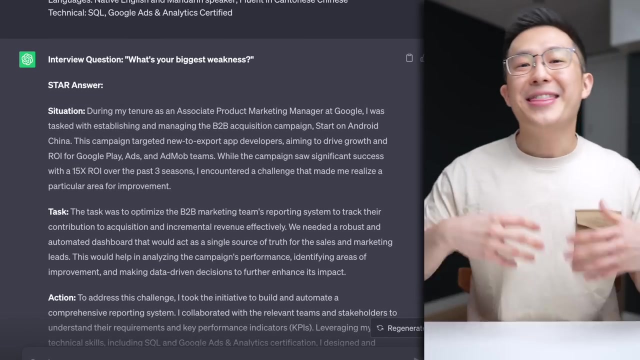 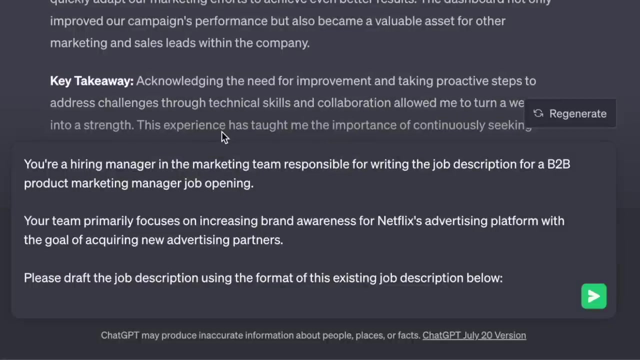 book titledander die opiates. Here, instead of using a full-blown interview answer as an example, which would be overkill, the star framework acts as an example structure for ChatGPT to follow. Last example: let's say you need to write a job description. 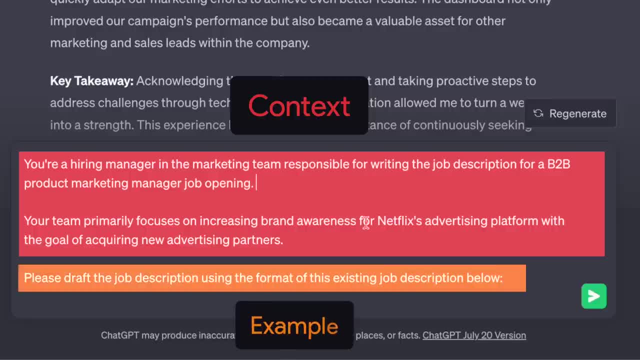 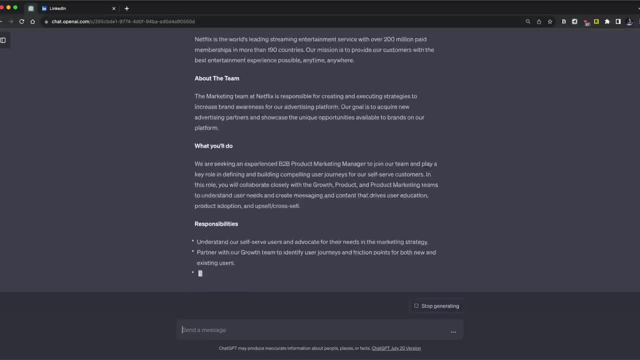 You give some context around the opening and ask ChatGPT to reference an existing job description. If I use this one I found on LinkedIn, the output will follow the same formatting and use the same professional HRE language, saving me a bunch of time. 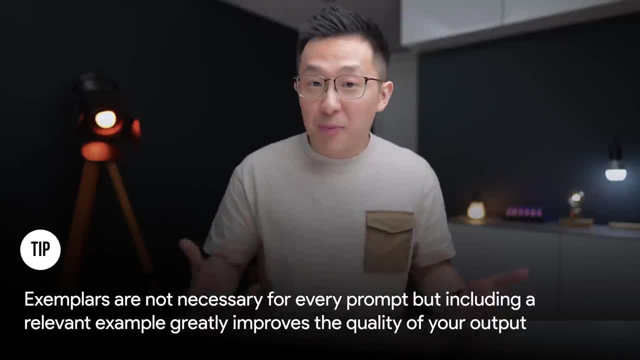 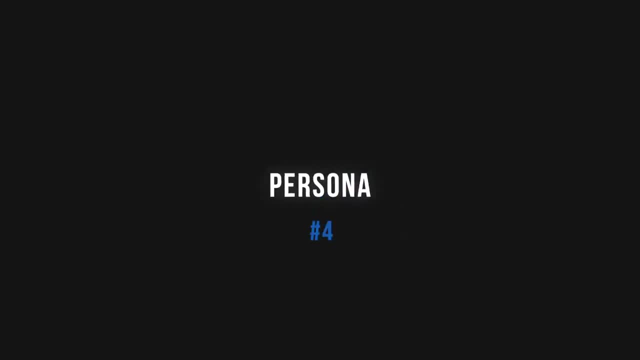 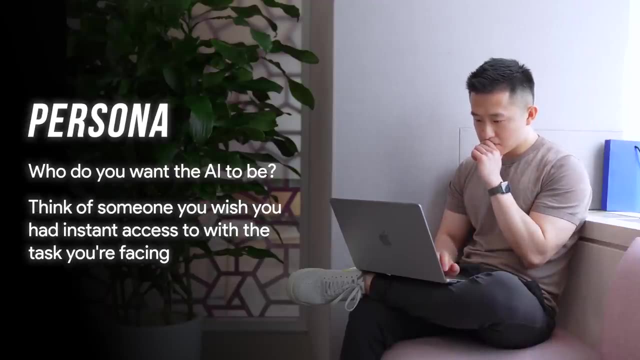 Main takeaway here: exemplars are not necessary for every prompt, but including a relevant example or framework will greatly improve the quality of your output. Moving along the persona component is basically who you want ChatGPT and BARD to be, And the pro tip here is that think of someone. 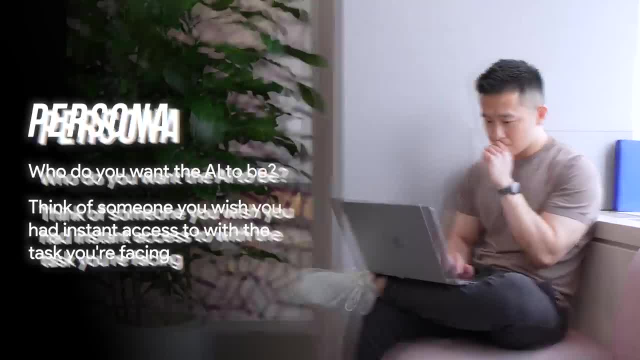 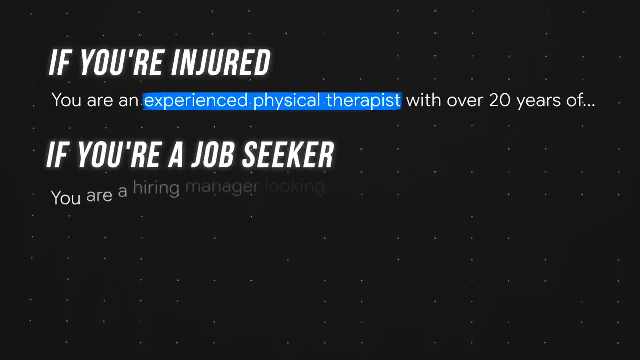 you wish you had instant access to with the task you're facing. If you injured yourself working out, that person might be a physical therapist with experience helping athletes recover. If you're a job seeker, that person might be a recruiter or hiring manager. 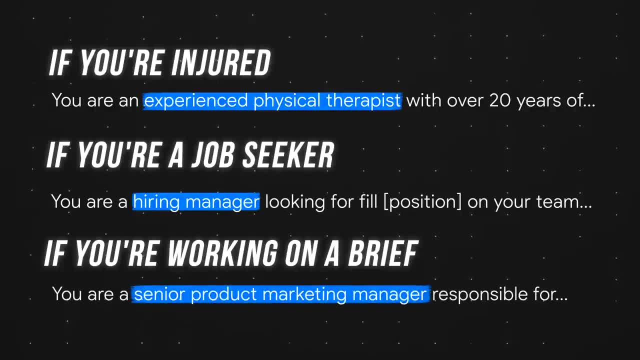 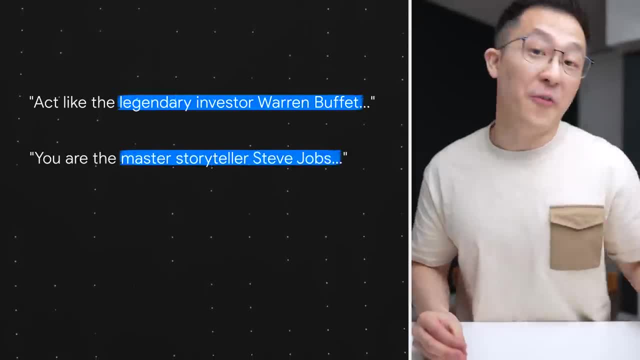 If you're working on a creative brief, that person might be a senior product marketing manager who's great at storytelling. Pro tip. I've also named specific individuals, but I found the results to be good only when they're famous enough, like Warren Buffett, Steve Jobs, Jeff Su. 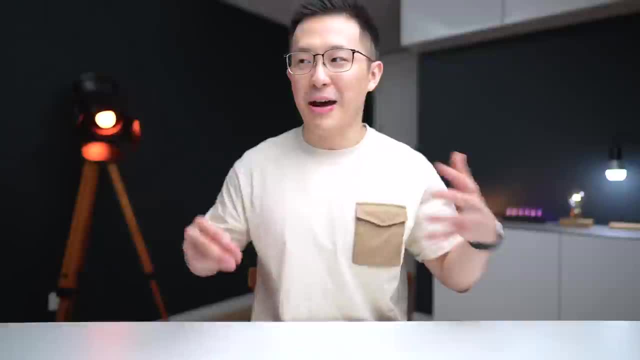 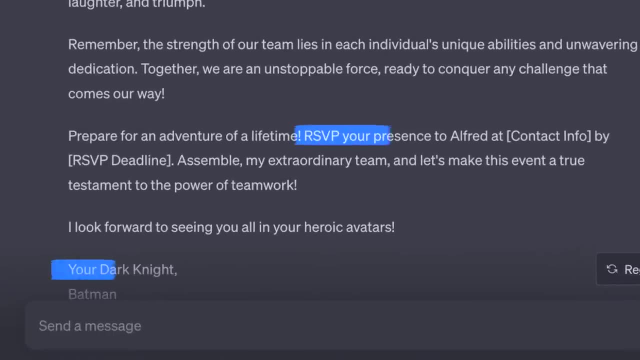 By the way, I just have to share this. We have a team offsite with a superheroes theme, So I asked ChatGPT to draft an email from Batman, and it even included things like: please let Alfred know and signed off as the Dark Knight. 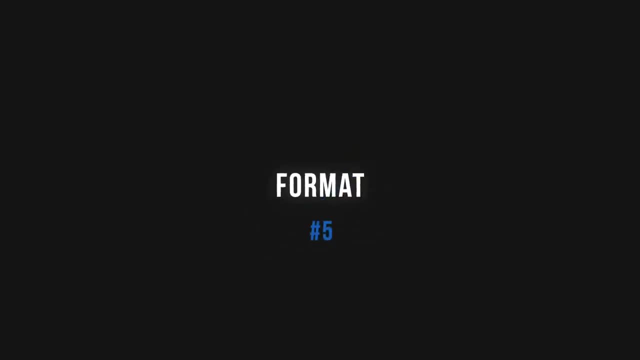 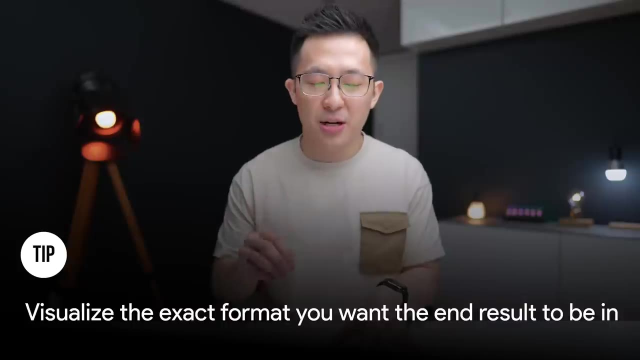 So fictional characters work as well, and I'm actually gonna use this, The fifth component format. The pro tip here is to literally close your eyes and visualize how exactly you want the end result to look. like A million likes on my thirst bomb Instagram photo. 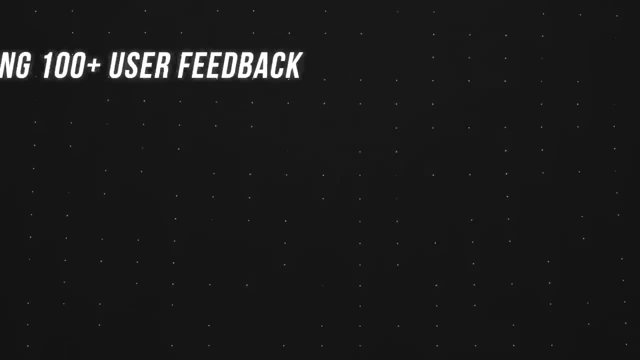 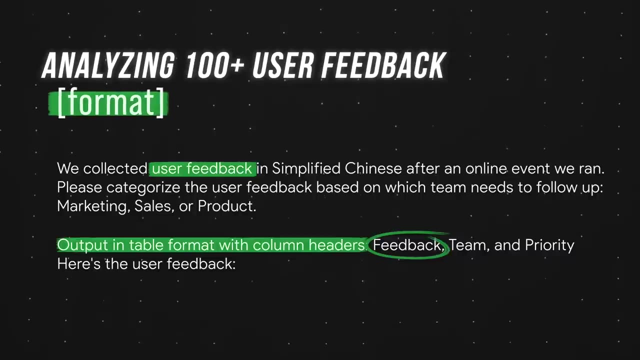 Dammit didn't work. Back to the user feedback example. I don't wanna read each sentence, So I asked ChatGPT to take all the feedback and output a table with three headers: The original feedback, the team responsible for following up and priority. 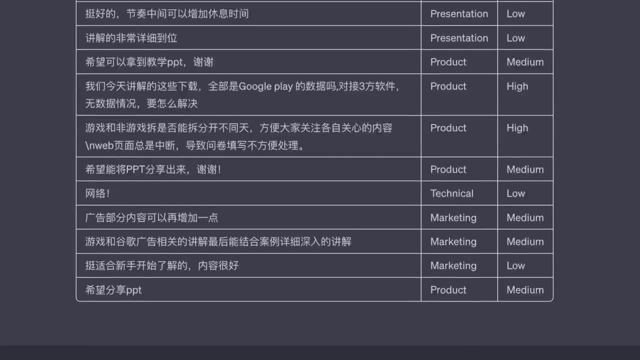 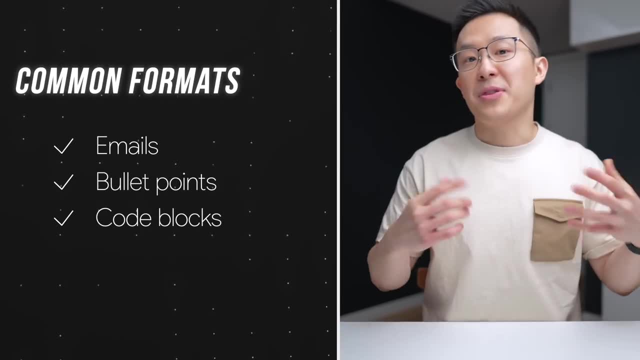 And now I can copy this directly and paste it into a Google sheet. So by priority and filter by team. Other common formats include emails, bullet points and code blocks, but the one I found to be the most useful is the one called the most useful as a full-time working professional. 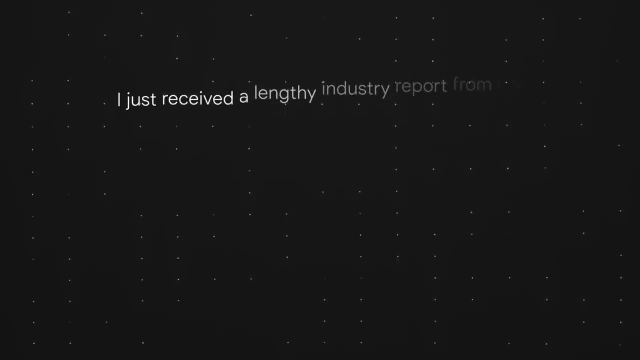 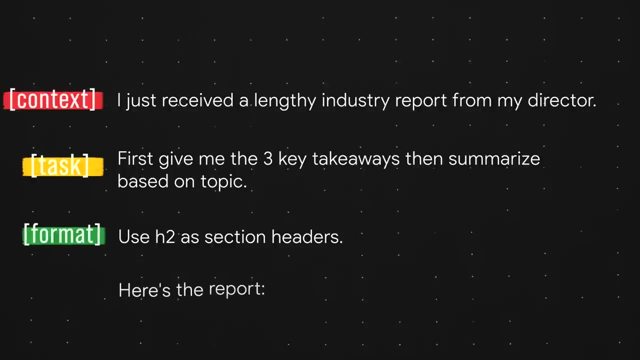 is paragraphs and markdown. For example, I just received a lengthy industry report from my director. First give me the three key takeaways and then summarize based on topic. Use H2 as section headers. Here is the report. Pro tip: whenever I use ChatGPT to proofread any document: 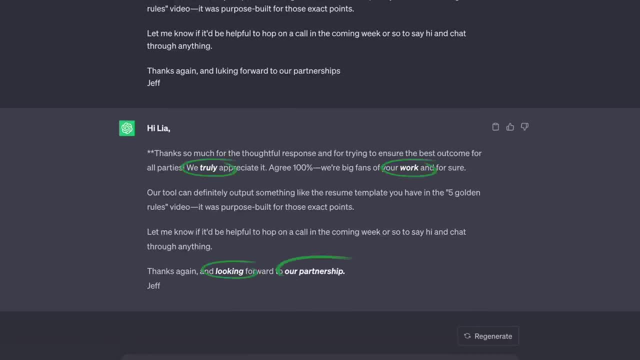 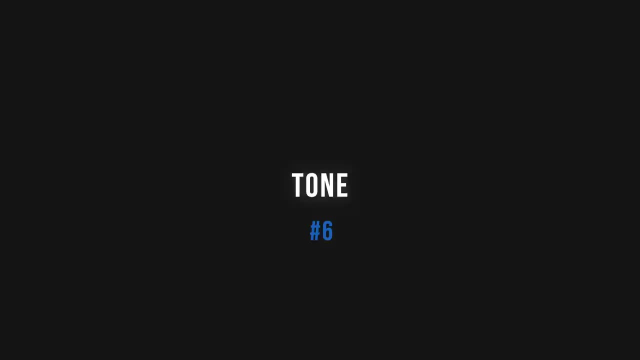 I specify that all changes need to be bolded so I can easily see exactly what has been changed. Let's quickly go through the last component, tone, before we put all this together in one example. The good news is, tone is easy to understand. 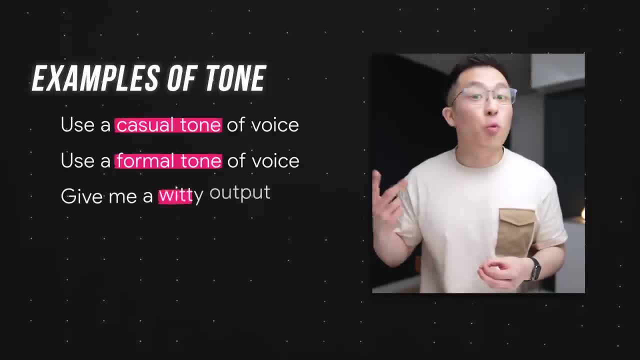 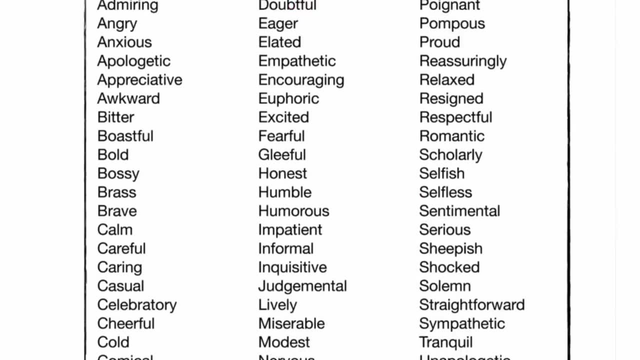 Use a casual or formal tone of voice. Give me a witty output. show enthusiasm. sound pessimistic. The bad news is we're usually not very good at recalling the thousands of potential adjectives and adverbs at a moment's notice. So here's a pro tip. 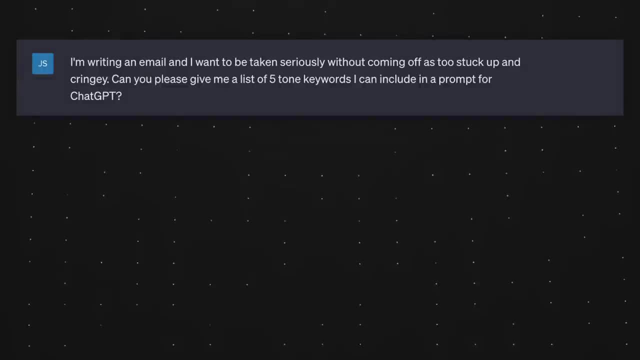 Tell ChatGPT the feeling you're going for. For example, I'm writing an email to a team I haven't worked with before and I wanna be taken seriously without coming off as too stuck up and cringy. Can you please give me a list of five? 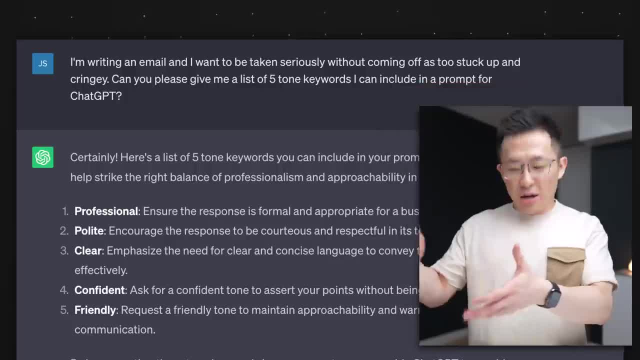 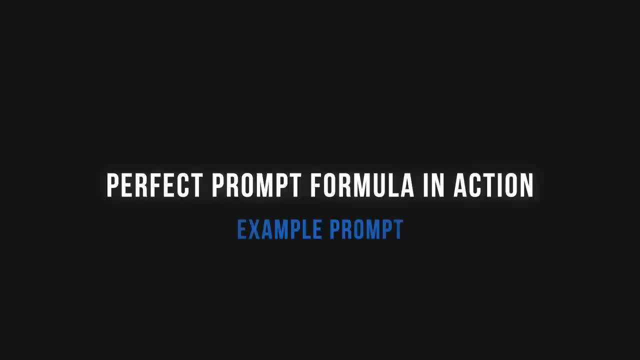 tone keywords I can include in a prompt for ChatGPT. And look now the actual prompt. I can say: use clear and concise language and write in a friendly yet confident tone. Putting all this together, let's look at this comprehensive prompt. 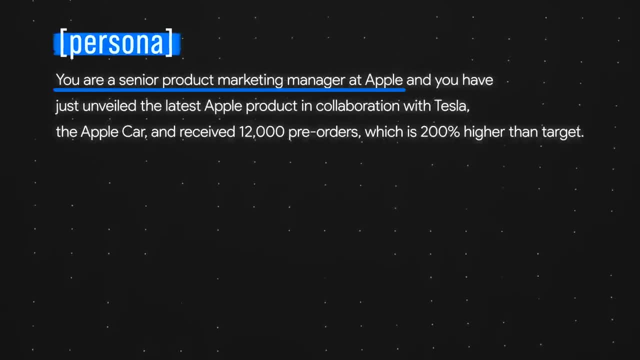 You are a senior product marketing manager at Apple persona and you have just unveiled the latest Apple product in collaboration with Tesla- the Apple car- and received 12,000 pre-orders, which is 200% higher than target context. Write an email to your boss, Tim Cookie. 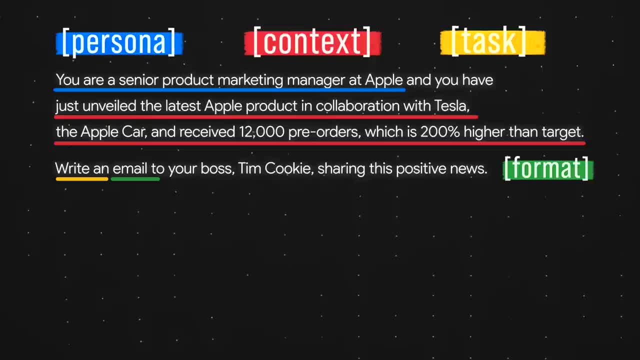 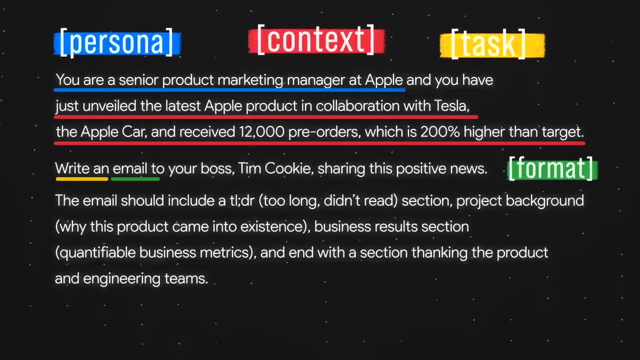 sharing this positive news. The email should include a TLDR. too long didn't read section: project background: why this product came into existence, business results section, quantifiable business metrics. and end with a section thanking the product and engineering teams. 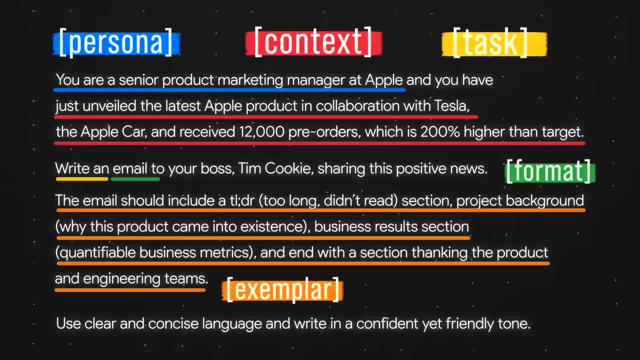 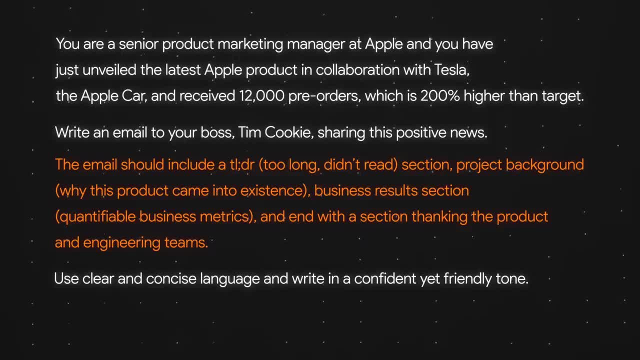 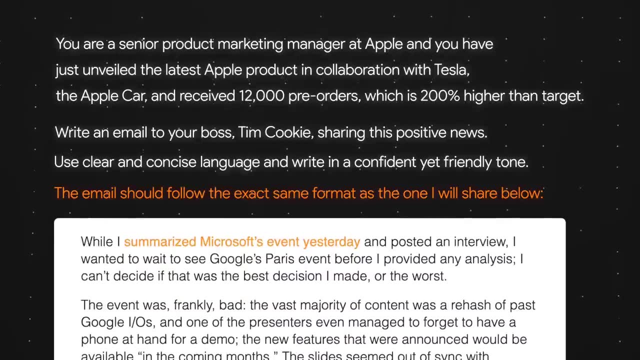 Example structure: Use clear and concise language and write in a confident yet friendly tone. Tone note that if I had an existing email to reference, I could delete the instructions around the structure and simply tell ChatGPT. the email should follow the exact same format as the one I will share below.